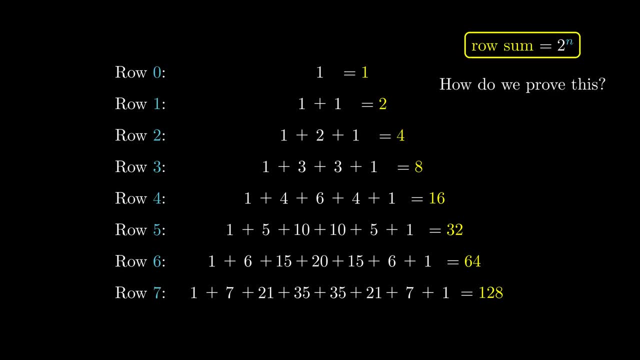 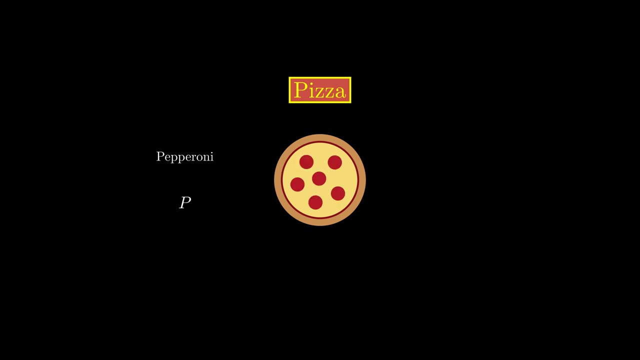 Now is the hard part. Can we prove this? Let's first propose a counting problem that at first may not seem related to this problem at all. Suppose I'm at the pizza shop and I'd like to buy one pizza. The pizza shop offers four toppings—pepperoni, mushrooms, bell peppers and sausage. 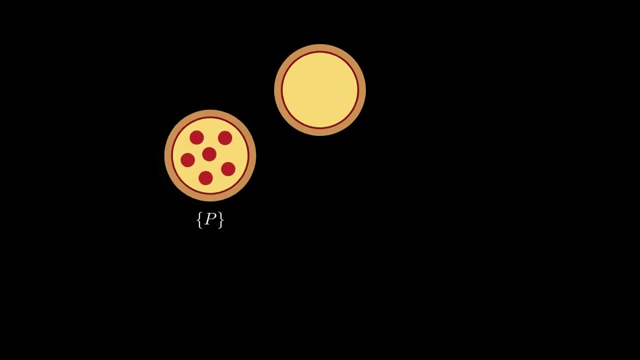 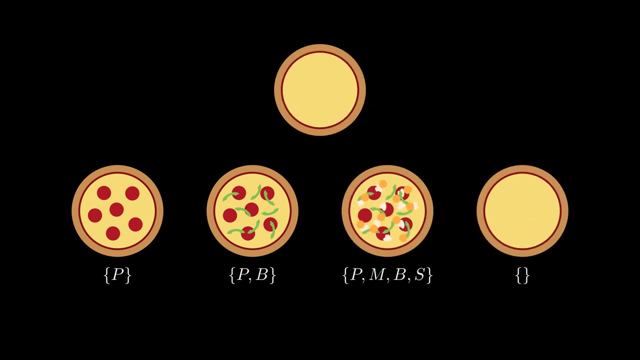 I can select any number of toppings for my pizza. I could choose a pepperoni pizza. I could choose a pepperoni and bell pepper pizza. I could choose all four toppings, or even a plain pizza, no toppings. How many different pizzas can I make? 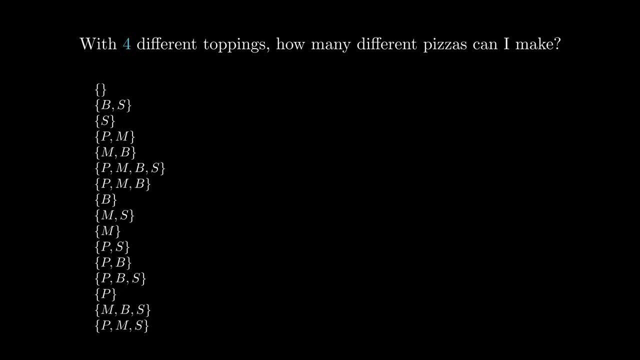 If you don't know where to begin, one thing you could do is start listing out some possibilities. Unfortunately, listing out the pizzas like this can be pretty annoying, because it's hard to keep track of all of them. If we wanted to count them in a more organized way, we should group or order them. 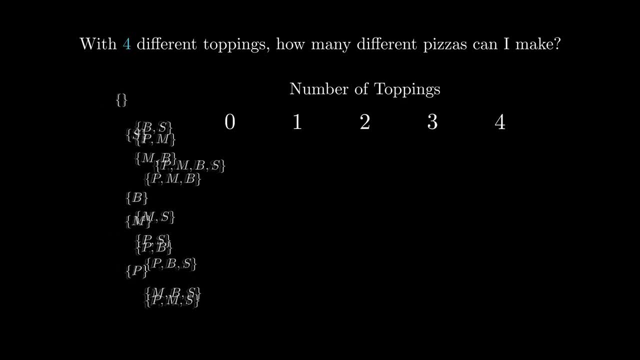 Let's group these pizzas by how many toppings there are. While I have all of the possibilities listed here, it's actually very easy to calculate how many belong to each case. For example, the number of ways to select two toppings out of four is simply 4, choose 2.. 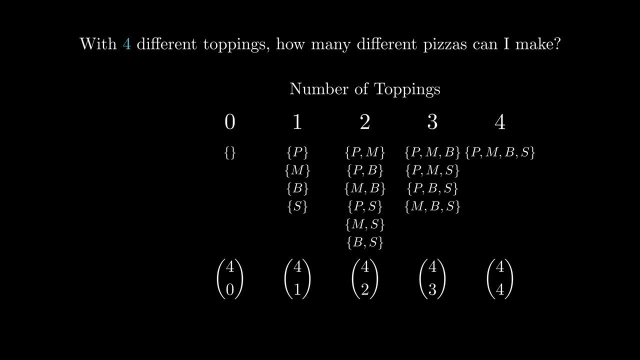 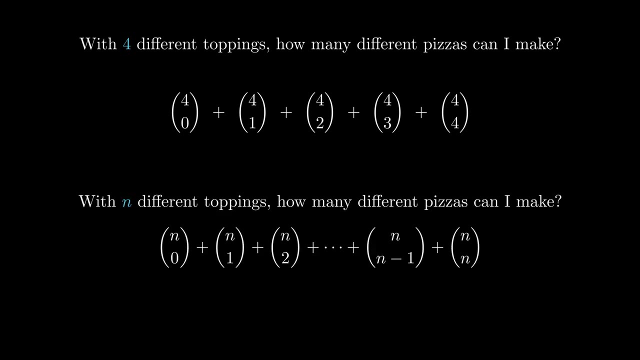 To find our total, all we need to do is add all of these combinations together. Here is our answer. It should also be easy to see that this solution is generalizable to an arbitrary n toppings. If we have n toppings, then this expression gives us the total number of possible pizzas. 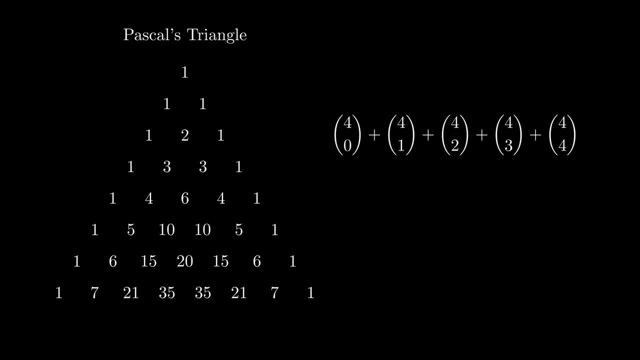 Now let's take a look at where each of these combinations are located on Pascal's triangle. 4 choose 0 is here, 4 choose 1 is here, and so on. Adding all of these values together adds the entire row of Pascal's triangles. If we want to add all of these values together, we need to add all of these. 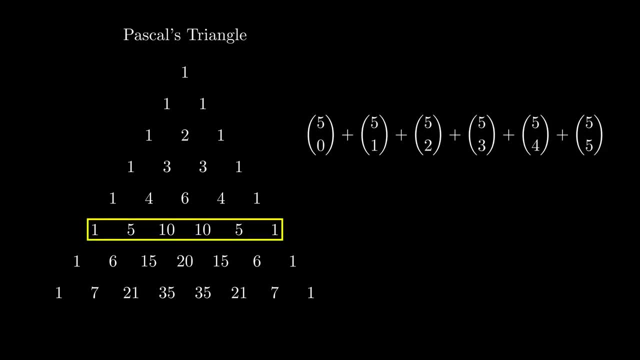 top volatilityStriple chakra as a middle form to the trinitial block In general. for n toppings, we would have to add up all of the values of Row n. Great, now we can see what this problem has to do with adding a row of Pascal's triangle, but we still haven't shown why. 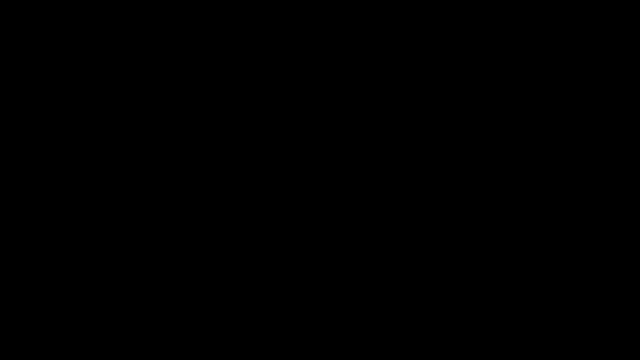 it's a power of 2.. Let's do that now. There's actually another way to solve this problem. Let's go through each of the toppings one by one. For each topping, I'll ask a simple question: Do you want it For pepperoni? you have two choices—yes or no. Step one is passing through each of the toppings one by one To select the topping that sunrise. in each of the toppings, either one will get the number, Level of spiceで. router For pepperoni. you have two choices—yes or no. 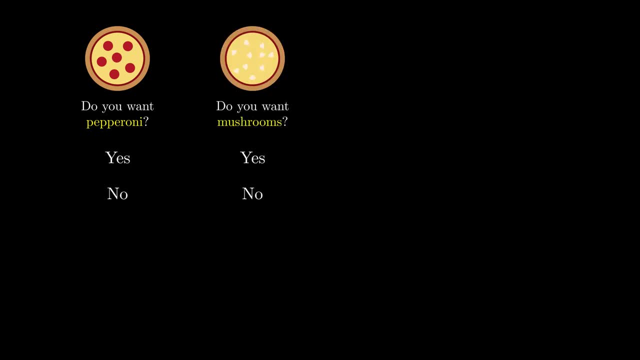 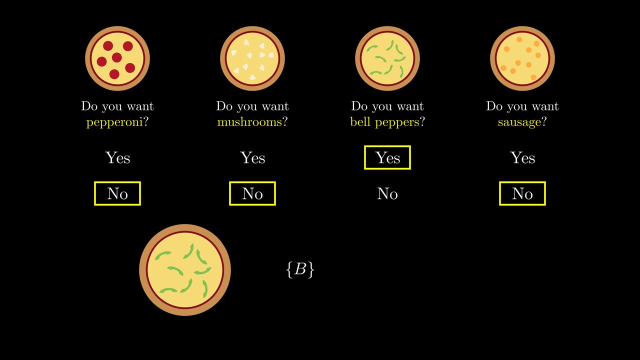 choices- yes or no. For mushrooms, you also have two choices: yes or no. Each topping gives you two options, and all of these choices together decide which pizza you want. Every pizza can be made in this way and every set of choices gives you a different pizza. guaranteeing that this is. 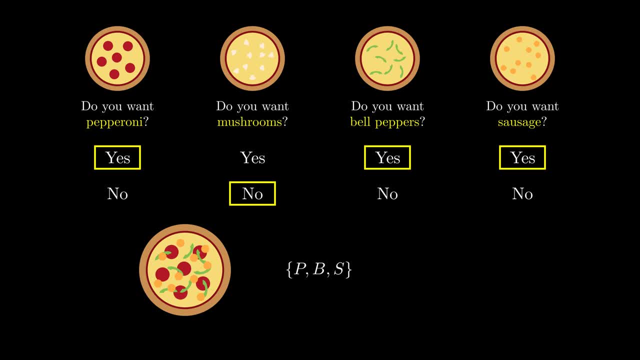 a way to construct the set of pizzas. How many pizzas are possible? now? Very simply multiply by two for each of the choices we have, giving us a grand total of two to the power of four pizzas. Again, it's easy to see that we can use the exact same logic to generalize this to n toppings. 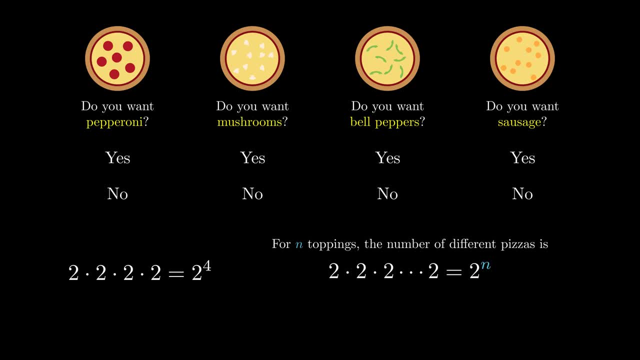 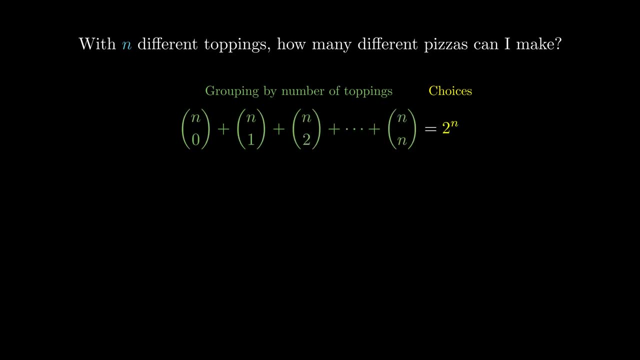 n toppings gives us two to the power of n possible pizzas. Since we solve the exact same problem in two different ways and the problem can only have one correct answer, both of these methods should yield equal results, proving that this expression, which we obtained from the set of choices, is the same as the set of choices. 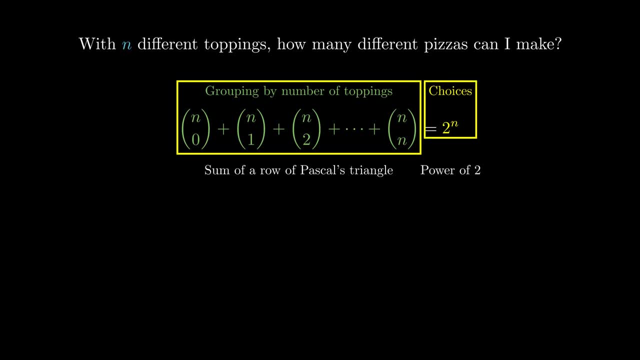 The expression we obtained from our first method and this expression we obtained from our second method must be equal. The left side is the sum of a row of Pascal's triangle, and this now proves that the sum is a power of two. This is called a combinatorial identity, because it is an identity. 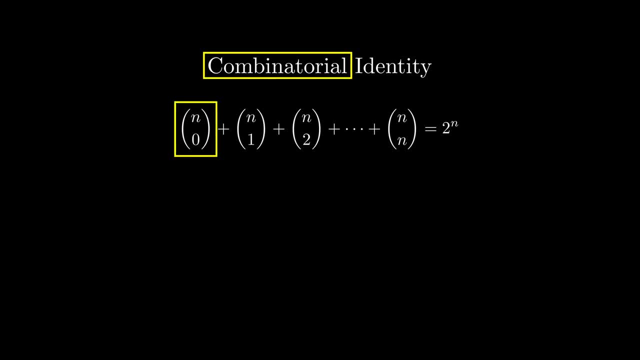 and it uses combination numbers. And the method of solving a problem in two different ways to prove a combinatorial identity is called a double counting proof. At first it was difficult to see why a row should add up to a power of two, But now let's look at the problem in two different ways. 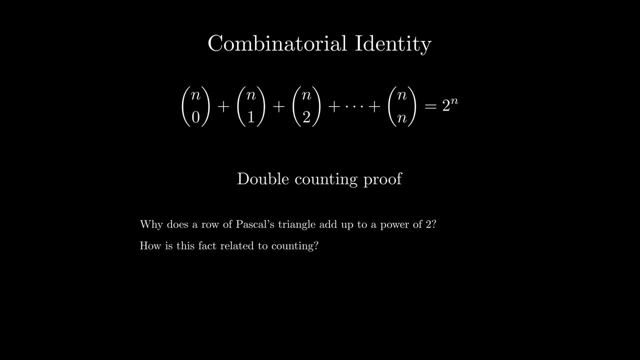 This particular counting problem manages to answer both of these questions at the same time. Isn't that cool. It turns out, however, that there is an even easier way to prove that the sum of a row of Pascal's triangle adds up to a power of two. Remember that to obtain the next numbers of 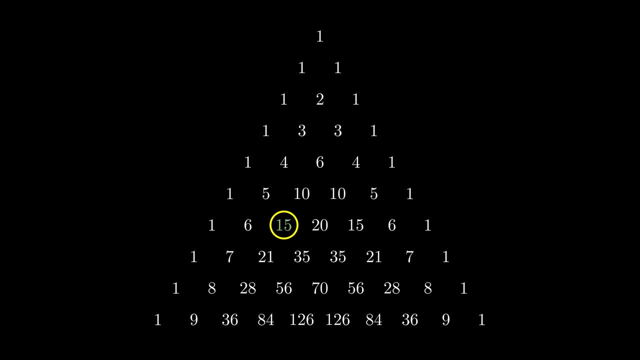 Pascal's triangle, we add the two numbers above each position. There's another way to think about this. We can instead say that each number in Pascal's triangle is added to both of the numbers below it. Look, this number is the sum of these two numbers. so it was added to the left And it 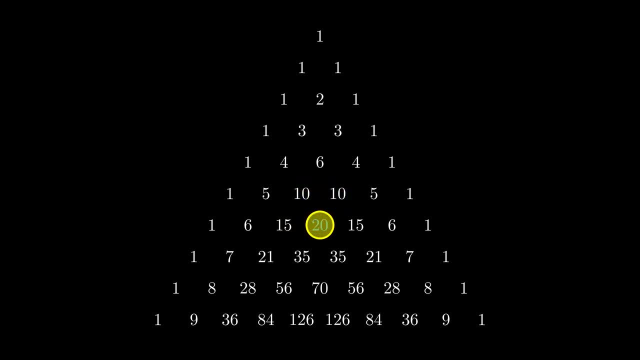 was also part of the sum here to its right. This is true for every single number in Pascal's triangle. If each individual number is added twice to the row below it, then wouldn't it make perfect sense that the row below is twice the sum of the previous row? Each time the number is added twice to the row below it, then wouldn't it make perfect sense that the row below is twice the sum of the previous row? Each time the number is added twice to the row below it, then wouldn't it make perfect sense that the row below is twice the sum of the previous row? 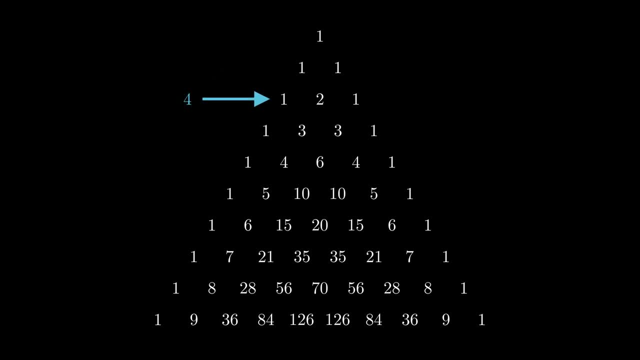 time you go down a row, the sum is multiplied by 2, which now easily follows that the sums are all powers of 2.. This is subjective, but I find this to be a much simpler proof, one that is very difficult to unsee once you've seen it. 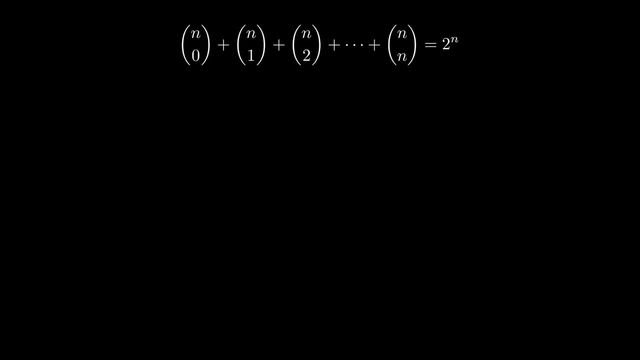 Almost like seeing how a magic trick is done, But just like a magic trick. even though how it works is now clear, I feel like some of the magic has been lost With the counting problem. it felt like we were drawing some meaningful connections to 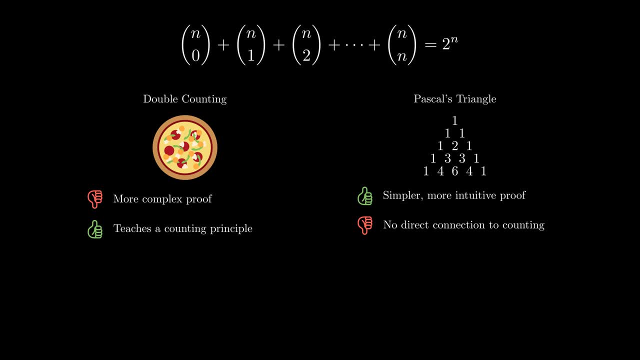 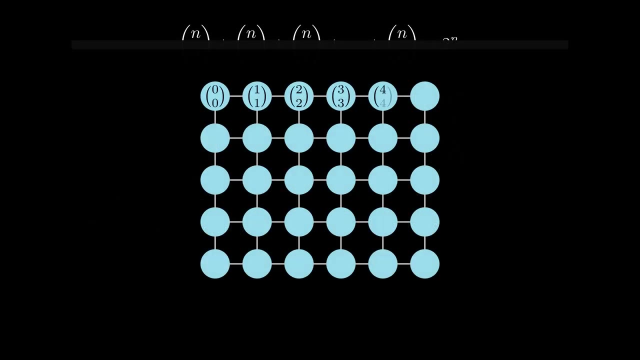 other problems, But here it seems like a very straightforward pattern. This is why I demonstrated the counting proof first. I wanted you to develop an appreciation for this pattern's connection to counting before explaining why this proof is also significant. Despite not having an immediate connection to counting, we still understand that this. 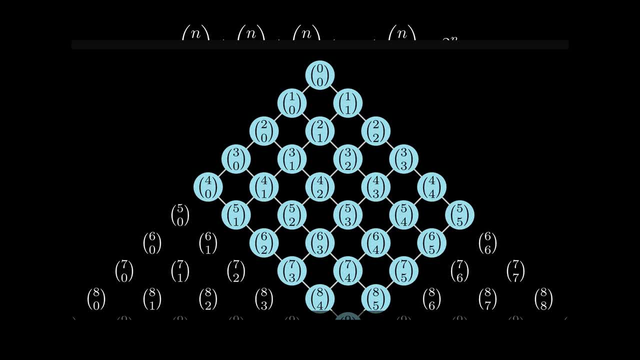 all abstractly and loosely still relates to counting, because all of the numbers in Pascal's triangle are still combination numbers. On top of trying to find a counterpoint to the problem, I wanted you to learn how to calculate the number of numbers in Pascal's triangle. 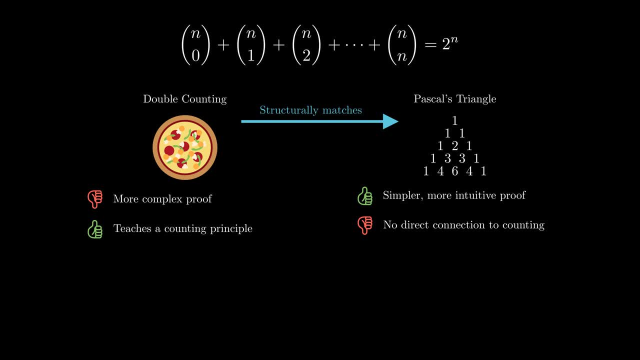 If we look at the counting application to Pascal's triangle, we can also think of Pascal's triangle as a tool that helps us see these counting relationships more easily. For this particular combinatorial identity, both the double counting method and the Pascal's triangle method are relatively simple. 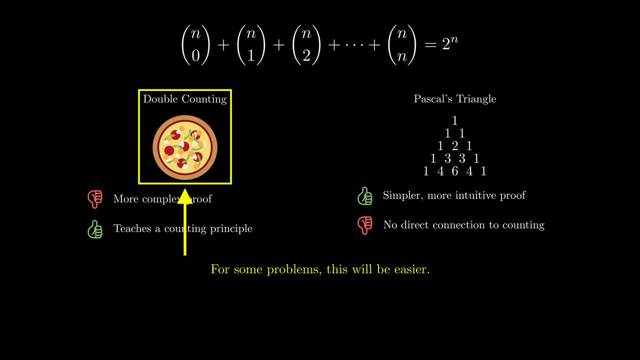 But there are some identities that are easy using double counting methods and hard using Pascal's triangle, or vice versa. The reason why they are so different is because the double counting method treats the numbers in Pascal's triangle as combination numbers And the Pascal's triangle method treats the combination numbers as numbers that are related. 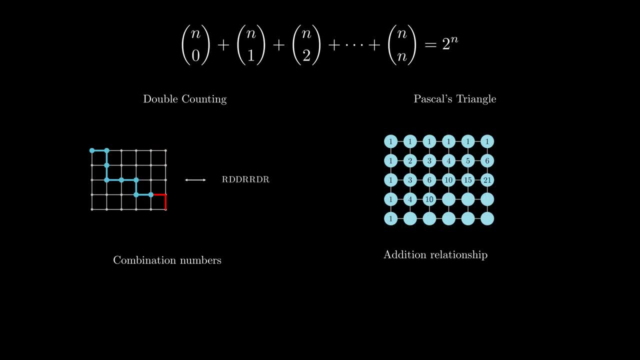 via addition. These are generally very different relational structures, so it's no surprise that they produce different approaches to a proof. Finally, there is a third way to prove combinatorial identities, and that just simply involves algebra. Remember that our combination numbers also had a formula involving factorials. 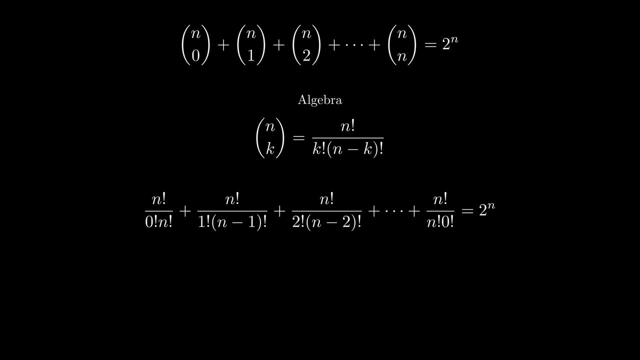 By simply plugging the values into the formula and simplifying we might be able to obtain a proof that way too. But if you actually try this method on this particular identity, you might find it is nearly impossible. This mostly has to do with a dot dot dot in the expression, which means you're adding. 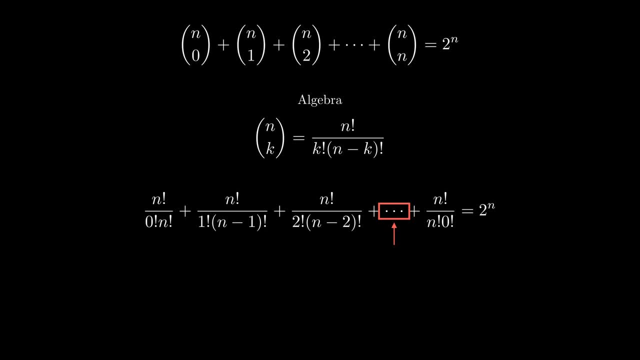 a variable number of terms, making it very difficult to simplify and combine. As usual, the algebraic approach isn't always difficult. For some problems, the algebraic approach will be far simpler than using double counting or Pascal's triangle. Each problem will be different. 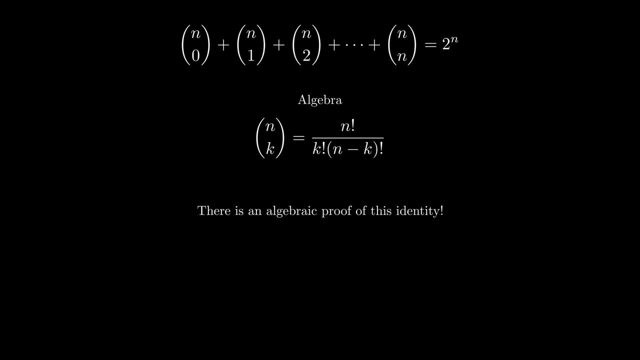 By the way, There is in fact a way to algebraically tackle this identity, but that I will save for another day, under a different context, to teach a different lesson. So what did we learn? As promised, we found one pattern within Pascal's triangle, related it to counting and proved. 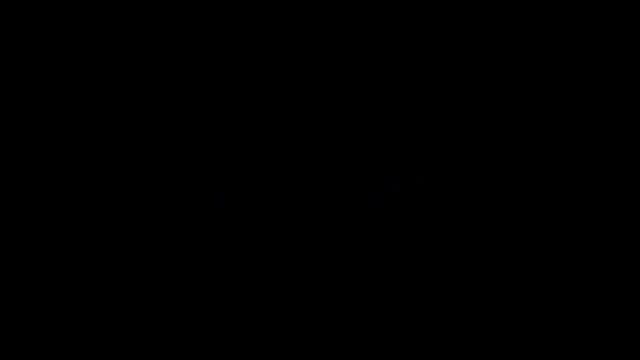 it. In the process, we learned to understand combination numbers in three ways: Combinatorially, by treating them as the number of ways to choose k objects out of n. Algebraically, by plugging in the formula And what I will call. iteratively or recursively, by visualizing their relationships on Pascal's 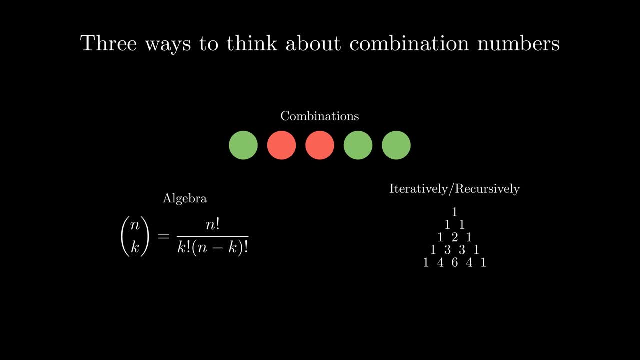 triangle. Whenever you're tackling a combinatorics counting problem, remember these three general ways to visualize your counting numbers. What may be difficult under one perspective could be much easier under another. I will be posting more videos going over lots of other patterns in Pascal's triangle with: 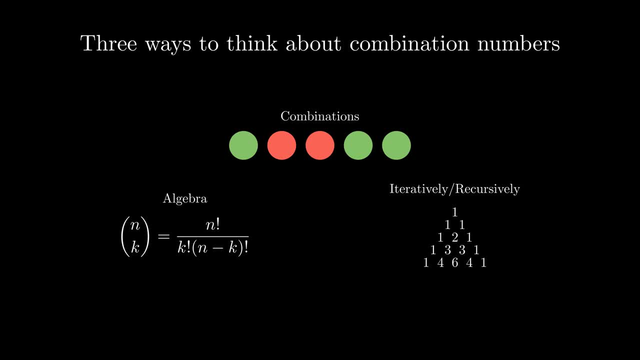 more examples of how to apply these ideas, But hopefully I've inspired your curiosity to explore. I'll see you in the next video, Bye-bye. What patterns can you find? Can you prove that these patterns work? What lessons does it teach about counting? 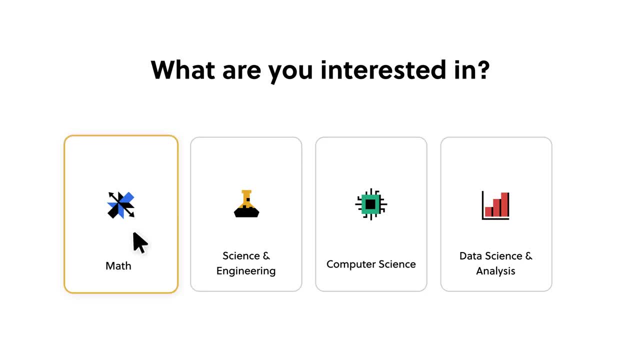 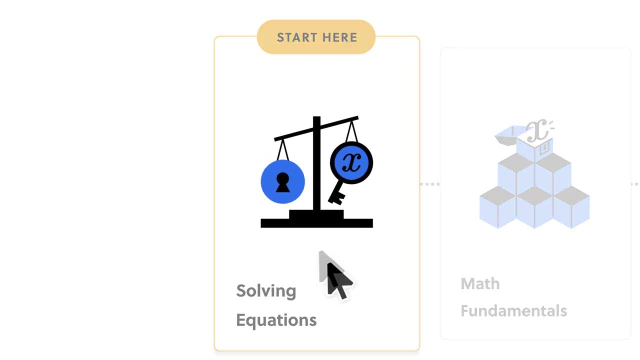 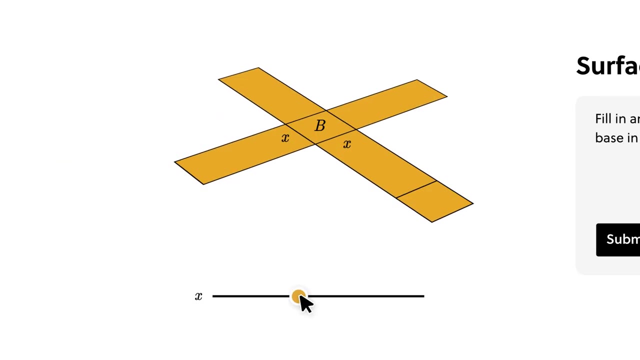 Watching a video abstractly outlining mathematical strategies can only get you so far, and that's why the sponsor of this video is Brilliantorg. Brilliant is a fun and interactive way to learn math, as well as data science and computer science, with thousands of lessons of various math topics at all levels, so you can solve. 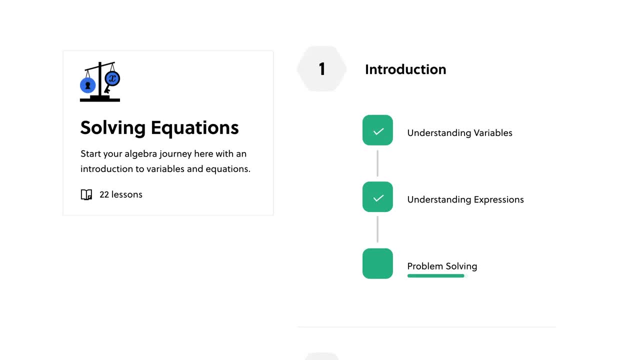 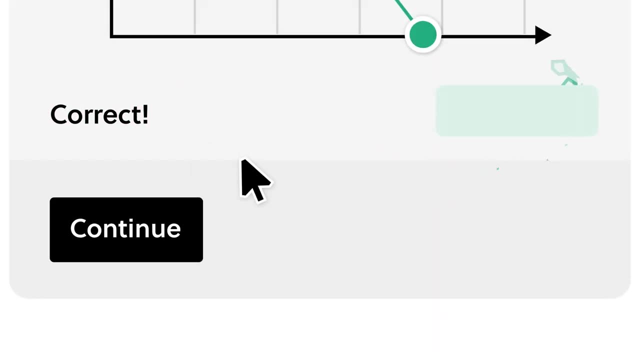 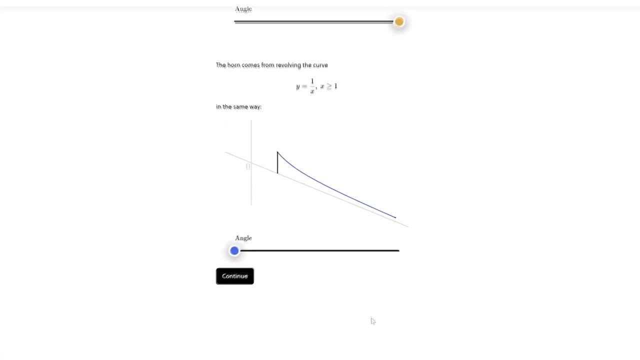 at your own pace And you can actually get some practice applying all of these ideas you've learned and testing yourself. Just as I try to use visual explanations in my videos, Brilliant provides not only visual but also interactive lessons. For instance, I enjoy this lesson that shows you what Gabriel's horn is, a shape that has.